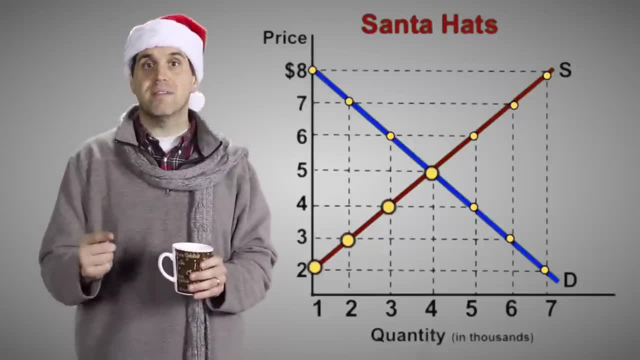 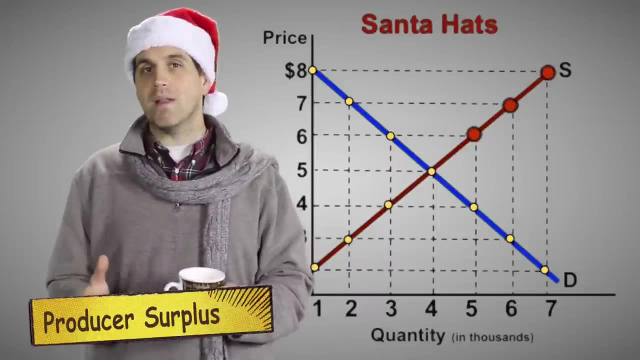 That's willing to sell hats for $2.. But every producer that's willing to sell hats for less than $5 makes producer surplus. It's the difference between the price and what a seller's willing to sell something for. But what about the producers that are willing to sell hats, but only if they can make more than $5?? 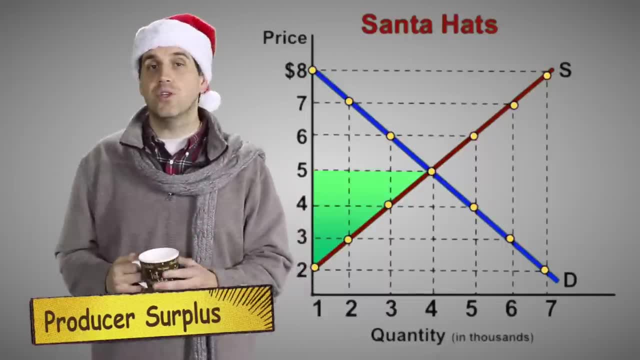 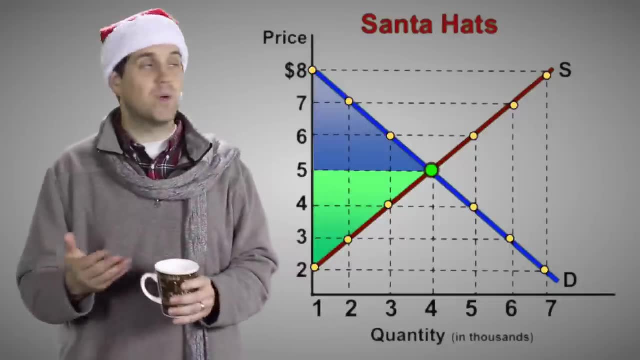 Well, they don't make a sale. Their costs are just too high. The combined producer surplus is the triangle right here, And so consumer surplus plus producer surplus, or total surplus, is right here. Now take a step back and look what's happening. 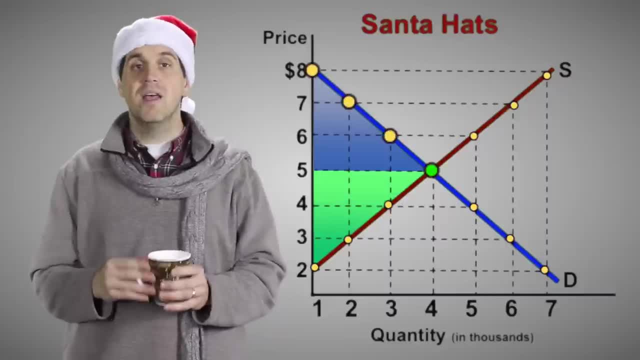 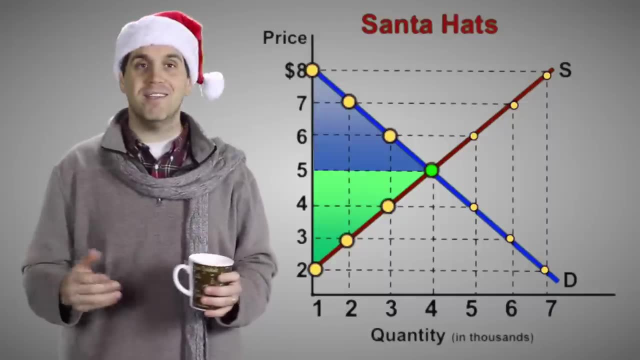 Markets are extremely efficient at allocating or distributing resources. The people who want Santa Claus hats the most get it, And they're made by producers with the lowest possible cost. That's awesome, Thanks markets. But what happens when a market's not at equilibrium? 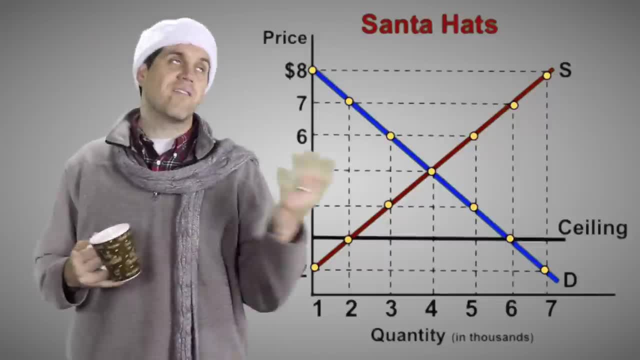 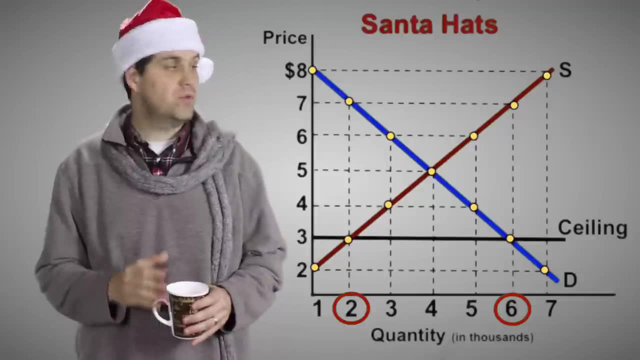 Well, let's say the government establishes a price ceiling at $3.. The government establishes a price ceiling at $3.. At that low price, consumers want to buy 6,000 units, But the producers are only going to produce 2,000 units. 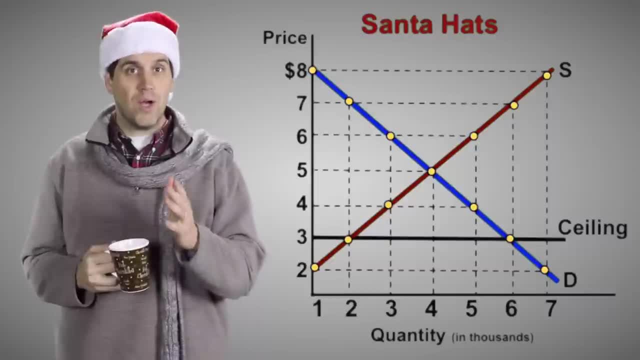 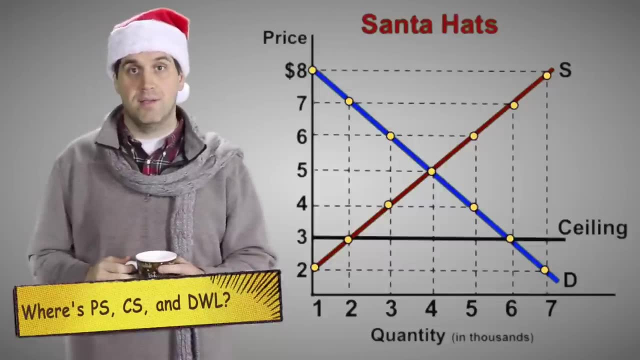 That's called a shortage and the result is deadweight loss. Now the question is: do you see it? Pause the video, see if you can figure out where's producer surplus, consumer surplus and this new thing called deadweight loss. 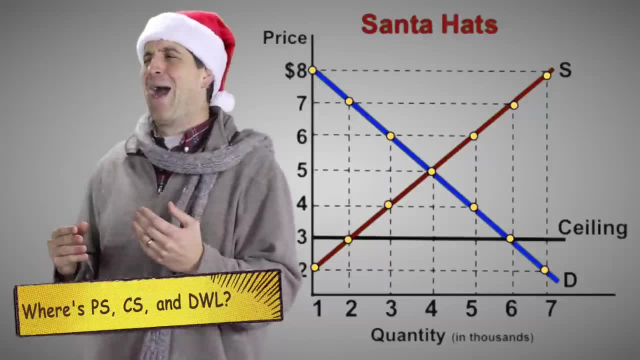 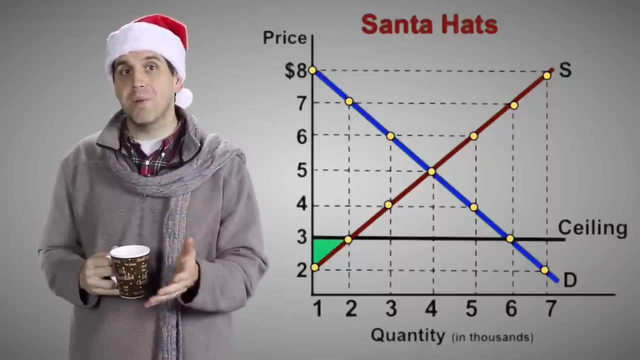 Play in the snow. Oh, gah, It's in my mouth. I totally missed you. Yeah, you did Okay. now that the price is lower, the producer surplus gets lower. It's right here. All the producers that are willing to sell above $3 are now out of the market. 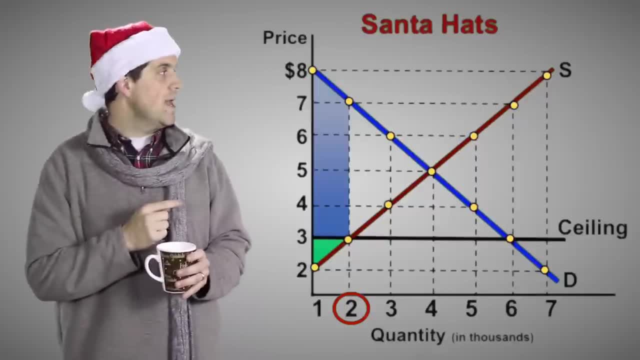 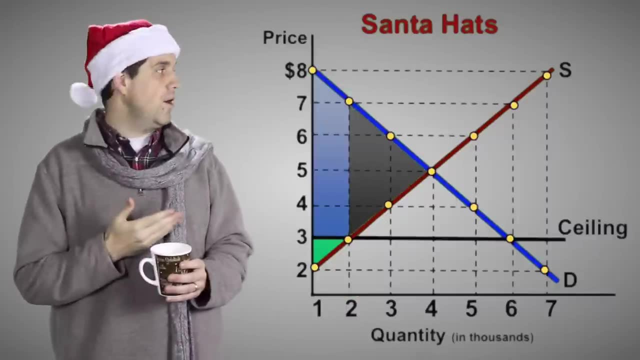 Since now there's no way to sell at $3. There's less output. The consumer surplus is right here. It's the difference between what consumers are willing to pay and what they actually did pay $3. That means the deadweight loss is right here. 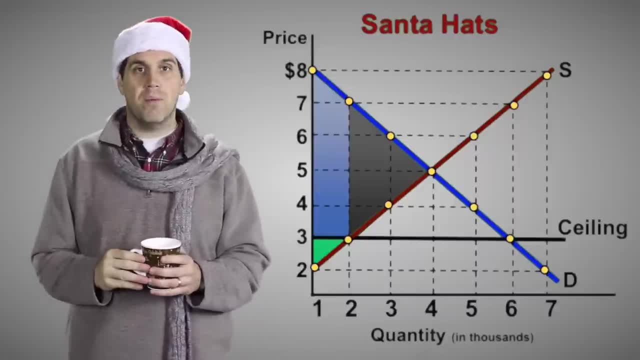 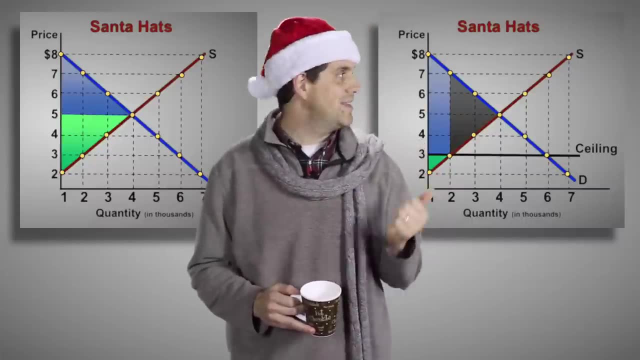 It represents the loss efficiency that occurs when the market doesn't reach equilibrium. We're not making the amount that society actually wants. When you compare the two markets- the one at equilibrium and the one with the price ceiling- you can tell that it's inefficient. 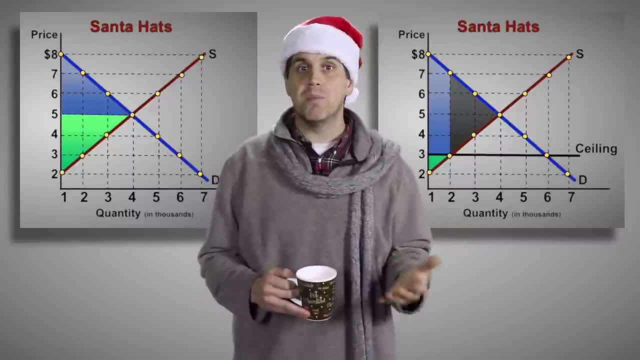 There's some consumer surplus and producer surplus that's missing, and so consumers and producers can benefit if we produce more output. Does it make sense? Okay, let's do it again, But this time let's see what happens when there's a price floor. 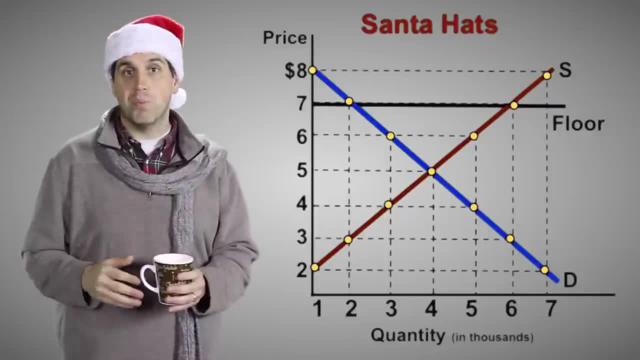 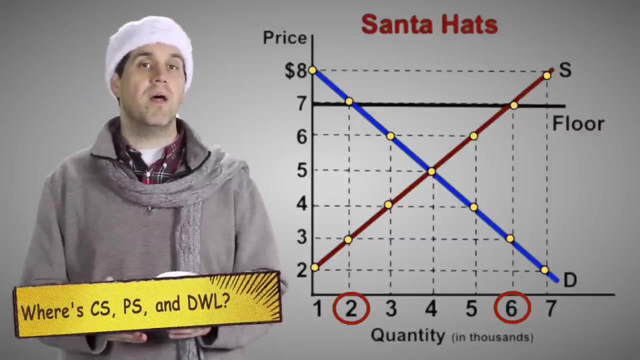 Now the government says the price can't go lower than $7, and the result is a surplus. Producers want to make 6,000 units, but consumers are only willing to buy 2,000 units. The question is: where's consumer surplus, producer surplus and deadweight loss? 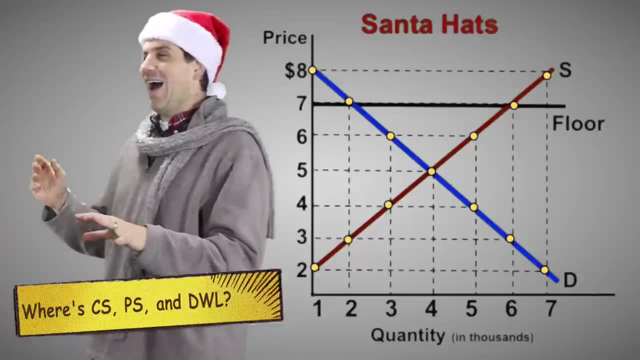 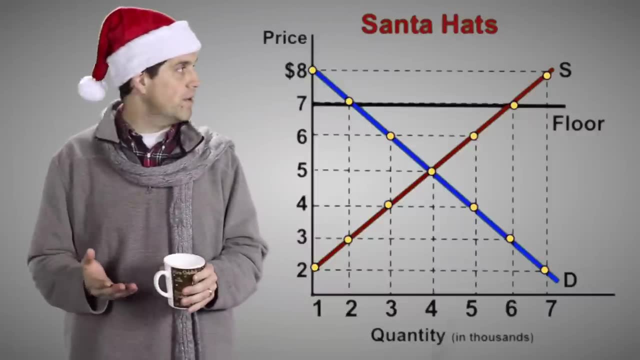 Playing the snow. Oh, you got me that time. All right. The price is higher, so consumer surplus becomes smaller. It's right there, And the producer surplus is right here. So right, there is the deadweight loss. Did you get that?